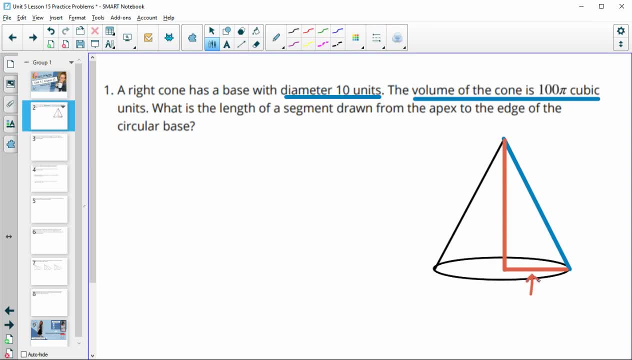 then we'll be able to find this blue one with Pythagorean theorem. So we know that the radius is five centimeters, since they gave us the diameter is 10.. So we're going to go ahead and first solve for the height so that we can go in and do the Pythagorean theorem. 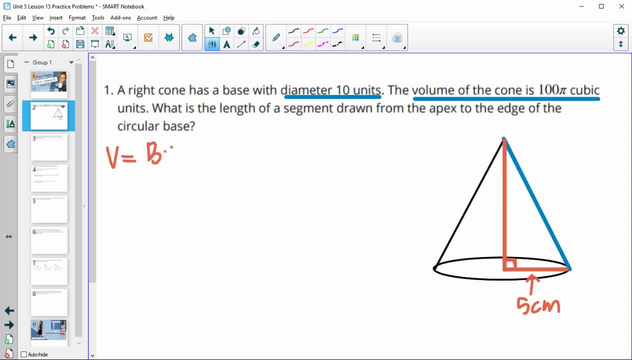 So for a cone the volume formula is area of the base times the height divided by three. They're giving us the volume is 100 pi And then they're giving us the base radius. So the area of the circle is the radius squared times pi. 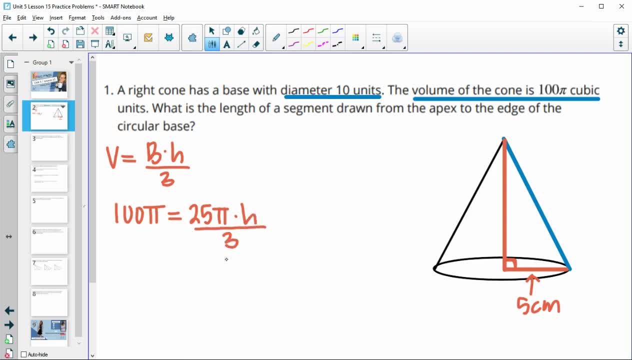 And then we have times H divided by three. So first thing I'm going to do is multiply both sides by three so that I can get this three off the bottom. So then we're at 300. pi equals 25 pi times eight. So now we'll be able to just divide by 25 pi. 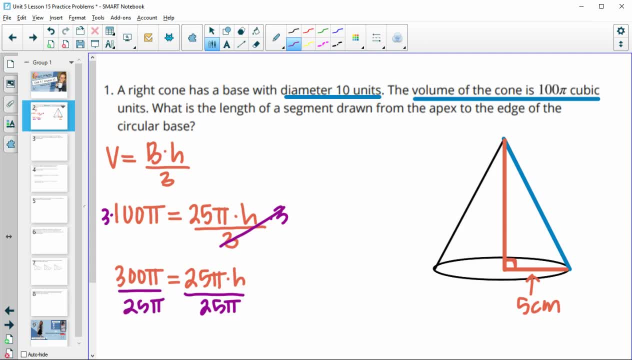 And that's going to give us our height. So when we, the those pi's, are going to cancel, So then we'll do 300 divided by 25 and we'll get 12 equals our height. So now we know that this is 12.. 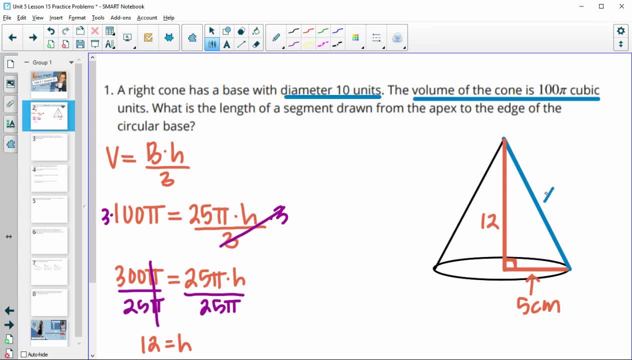 Then we'll be able to do Pythagorean theorem to figure out this length, And so we'll have: X squared is equal to 12 squared plus five squared. So X squared is equal to 144 plus 25.. Which is 169.. 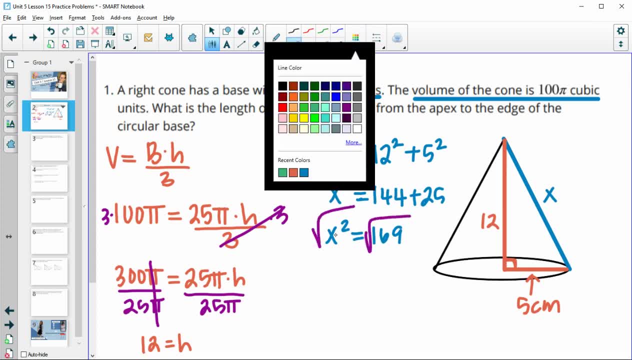 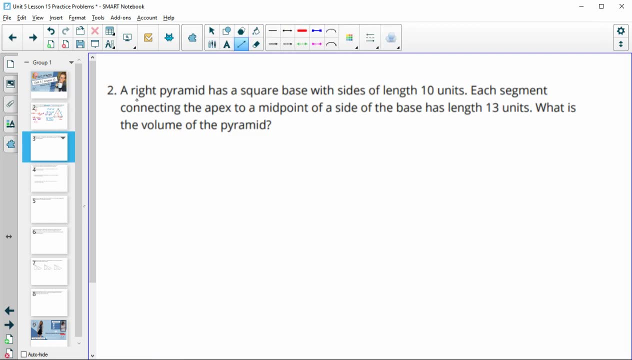 And then we will square root and get that X is equal to 13 units. Number two: we have a right pyramid with a square base. So there's our shape. It has side lengths of 10.. So the square base has side lengths that are 10 units each. 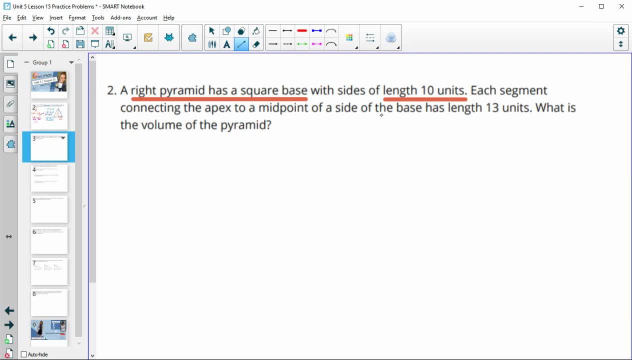 Each segment connecting to the apex to the midpoint of the side of the base has a length of 13 units. What is the volume of the pyramid? So let's go ahead and draw out This pyramid. Okay, so let's get the square base here and then going up to a point, 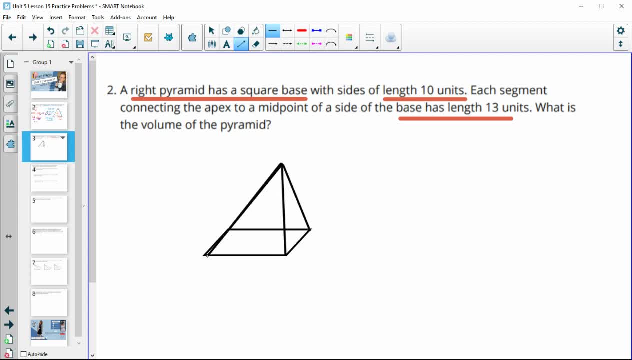